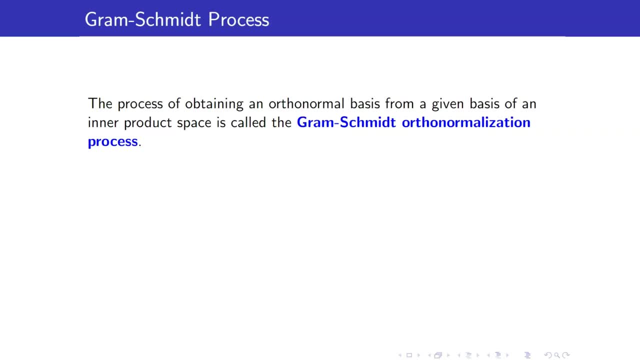 is what we call the Gram-Schmidt orthonormalization process. This process has three steps. First, we begin with a basis for our inner product space. We then convert it into an orthogonal basis And the last step is to normalize each vector to form an orthonormal basis. 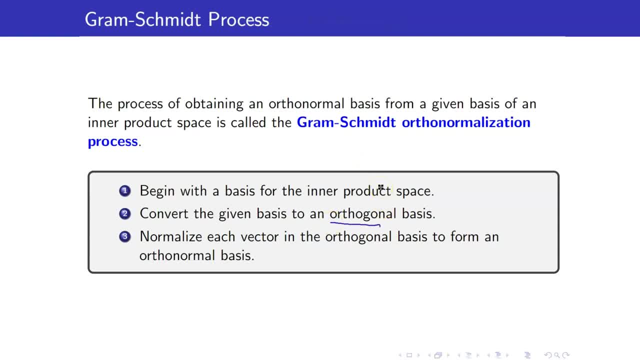 Notice that you can actually stop here in step 2 if you just want to get an orthogonal basis. But of course the nice thing with having an orthonormal basis is remember that when we write a vector W as a linear combination of the basis elements. 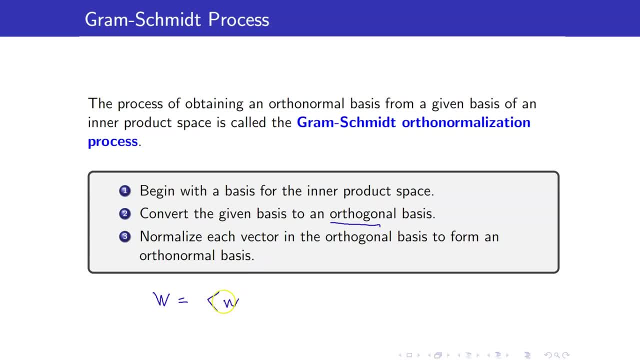 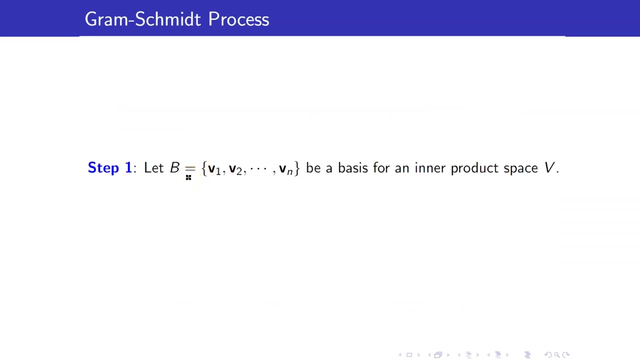 wherein our basis is a vector, the coefficients will just be the inner product of W, with the basis elements in your orthonormal basis, Correct. So that is why we want to turn all of our bases into an orthonormal basis. Here is our first step. 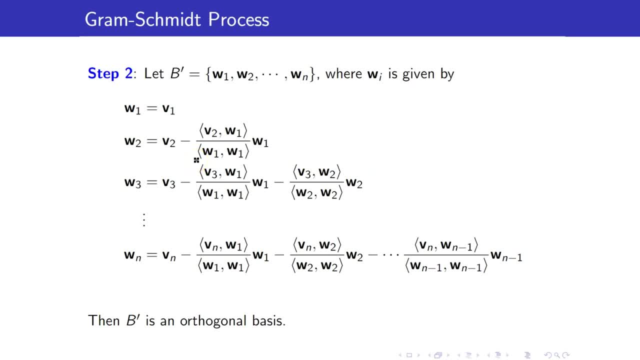 We begin with our basis And then we now define B' As follows: The first vector is just the original vector that we had. We call that. our B is V1, up to Vn Now to get W2, the second vector. 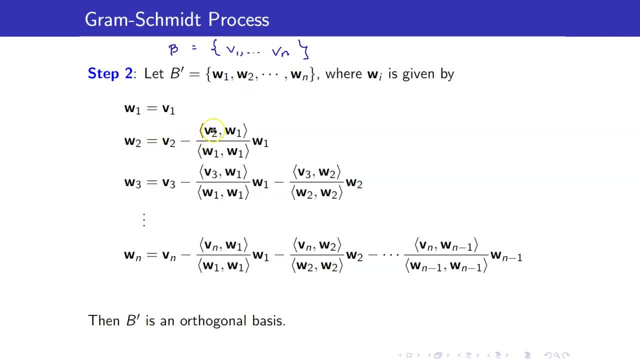 it's equal to V2 minus the inner product of V2 with W1 over. this is the length of W1 squared times W1.. W3 is V3 minus. you get the inner product of V3 with W1 over, the length, again, of W1 squared times W1, and so on and so forth. 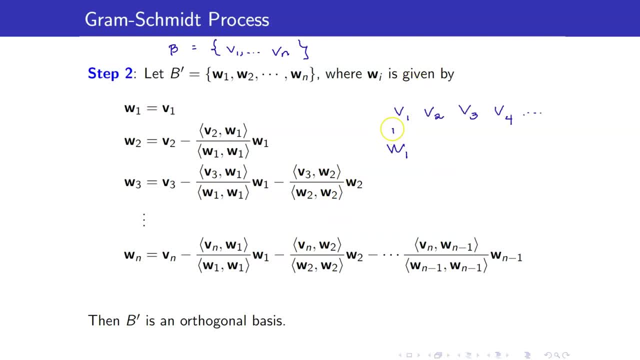 So basically, what's happening there is, we started with having W1 equal to V1.. For W2, it's equal to V2 minus the inner product. when I put my arrow here, it's the inner product of V2, with W1 over. 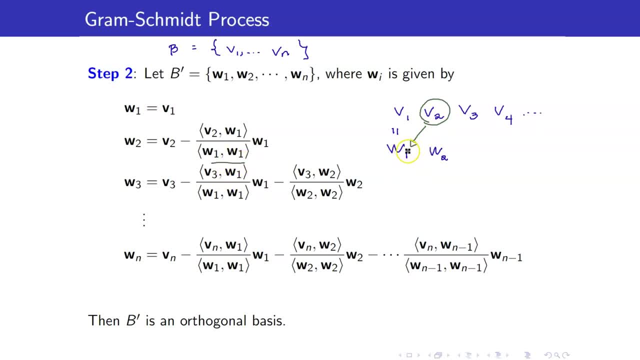 the length of W1 squared times W1. When I want to go to W3, it's equal to V3 minus inner product of V3 with W2 over the length of W2, squared times W2 minus the inner product of V3 with W1, and so on. 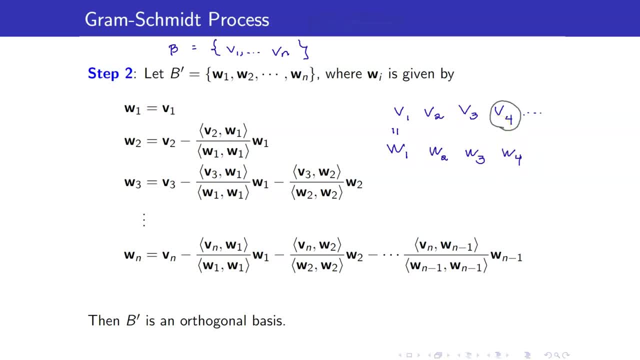 For W4, you start with V4 minus inner product of V4, with W3 and so on. You do that. you get the inner product of this vector. with these vectors, If we define our WIs as follows and we collect all of them in a set, 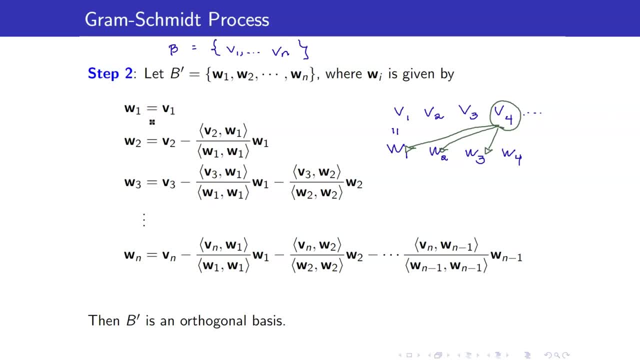 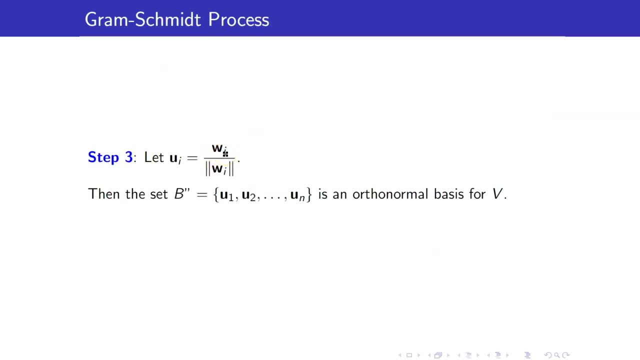 then that set will form an orthogonal basis. Then for step 3, we just normalize each of the vectors that we obtained in step 2. to get an orthonormal basis for V, For example, let us apply the Gram-Schmidt. 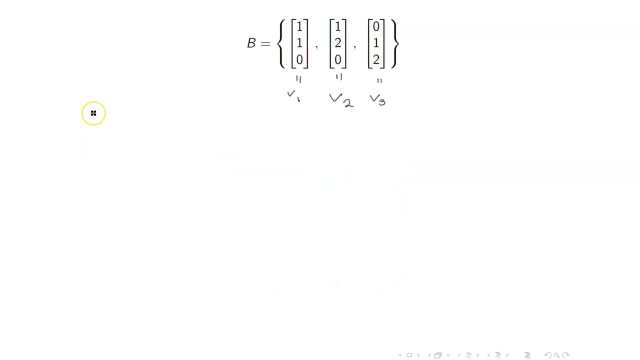 orthonormalization process, We now turn this into an orthogonal basis. W1 is the same as V1.. Next, W2 is equal to V2 minus inner product of V2, with W1 over the length of W1 squared times W1.. 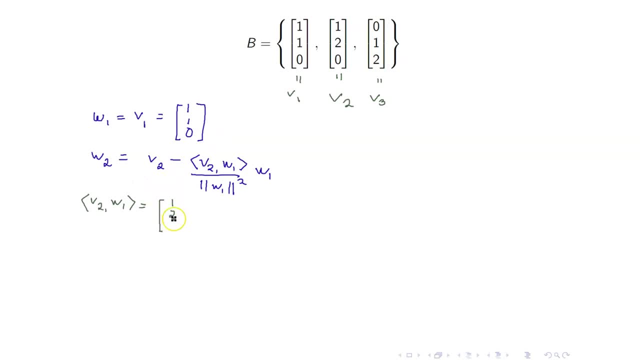 V2. W1 is the dot product of 1, 2, 0 and 1, 1, 0. So this is equal to 1 plus 2, so that's 3.. W1 squared, that's V1.. 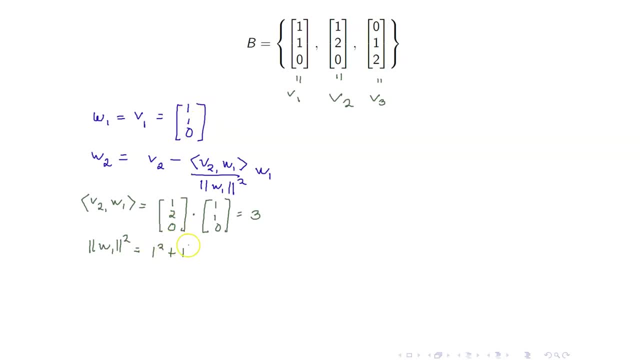 So that's 1 squared plus 1 squared, we have 2.. So therefore our W2 is equal to V2, 1, 2, 0, minus 3 halves times W1. This is equal to negative 1 half 1, half 0.. 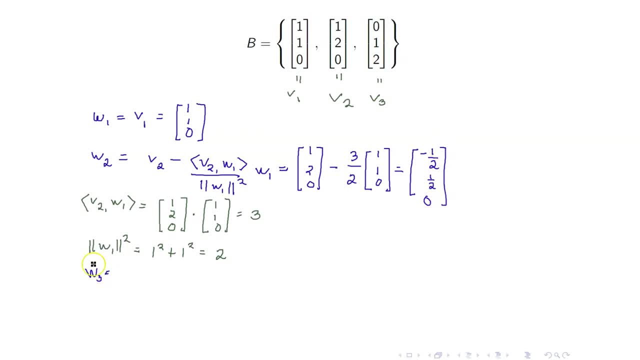 Next, let us get our W3. W3 is V3 minus. get the inner product of V3 with W1, then V3, W2 times W2.. Let us evaluate V3, W1.. So that's 0,, 1, 2, dot product with W1, which is 1, 1, 0.. 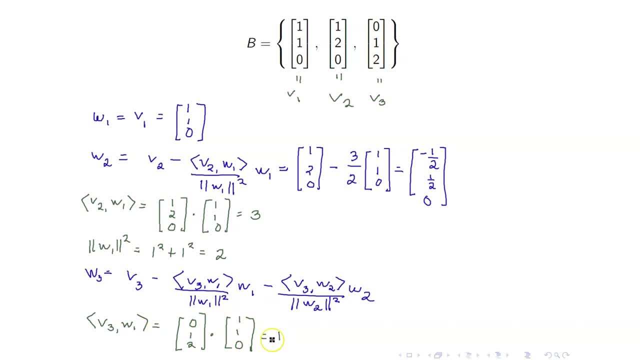 This is equal to 1.. What else We want? V3, W2.. This is equal to 1 half T. So let us now substitute: This is: V3 is 0, 1, 2 minus V3, W1 is 1. 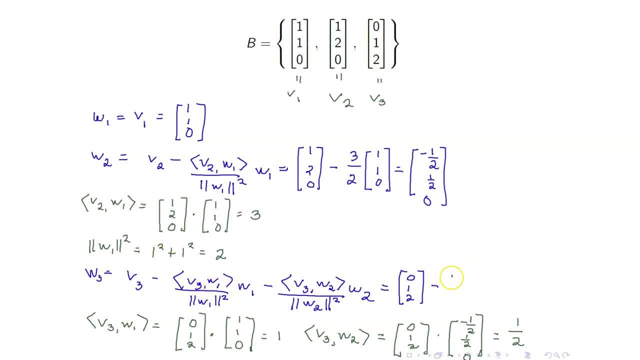 and then W1 squared. the norm is 2 times W1 minus v3 w2, that's one half over the norm of w2 squared. verify that the norm of w2 squared is also equal to one half times w2, which is negative: one half, one half zero. upon performing this. 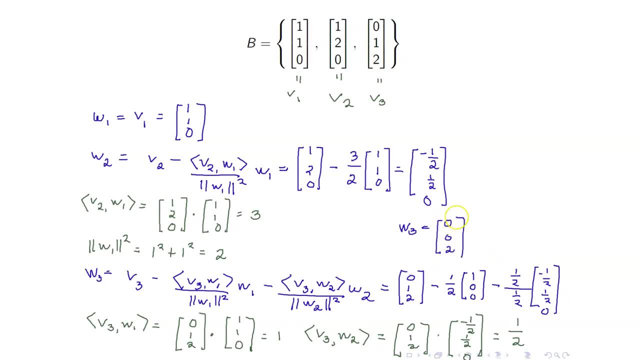 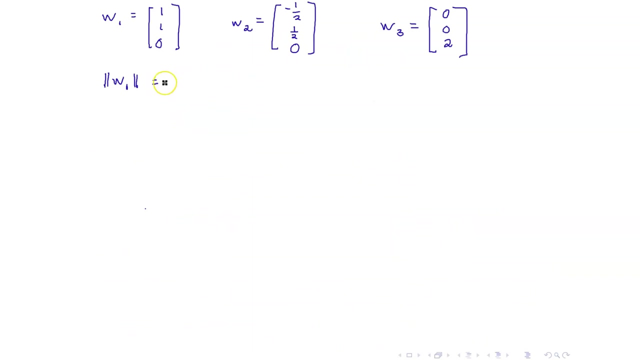 operation. this will turn out to be zero zero two. so here are our w1, w2 and w3. these three vectors will form an orthogonal basis. let's now turn this into unit vectors. to get an orthonormal basis, let us compute for the lengths of each vector. we have already computed that. the length of w1. 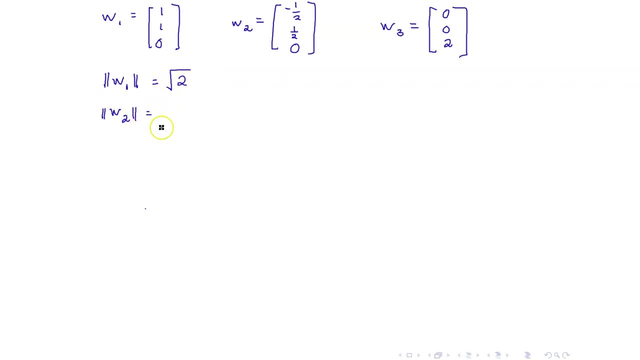 is square root of two. the length of w2 is the square root of one-fourth plus one-fourth, so that's one over square root of two. and the length of w3 is, of course, the square root of two, squared, which is equal to two. our u1, which is w1. 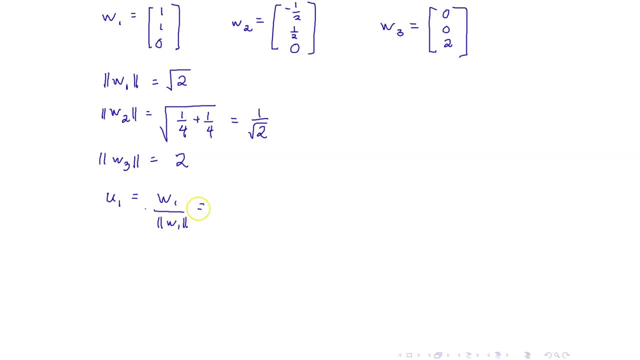 over the length of w1 is now equal to one over square root of two, one over square root of two- zero. our u2 is negative square root of two over two, square root of two over two zero. and, lastly, our u3 is equal to zero zero one. these three elements will now be our orthonormal basis. 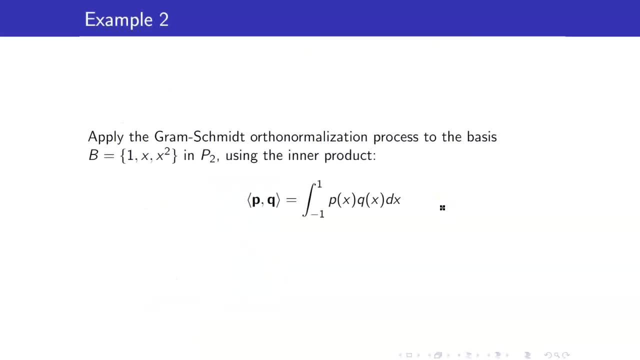 here's another example of an orthonormal basis. let's now compute for the length of w1, w2 squared. let us apply the gram Schmidt orthonormalization process to this basis. so remember also that the gram Schmidt orthonormalization process will always depend on the inner product, that is. 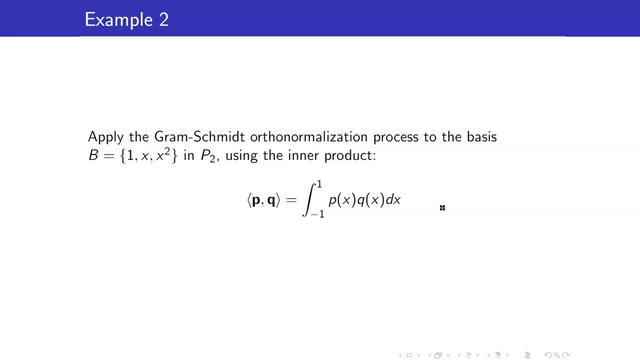 defined on your vector space. so in this case the inner product of two polynomials, PQ is defined to be the integral of P of X times Q of X, from negative one to 1. so let's proceed. let us first compute the volume. one double u, one is just theалы sort of, and the future state constant is just always power a minus Maori basic. so w1 equals Piece squared, timeswind Gibbs squared. so let us compare. and E two half squared by contract, negative one times placed, order ofarta normalize. and L squared equals P a minus解, square root of Px. no إلى Ay by loop. 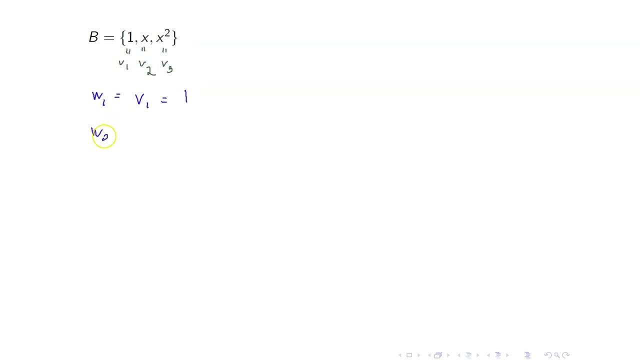 is equal to v1, so that's 1. w2 is v2 minus the integral of v2 with w1. all over w1 square times w1. let us compute the inner product of v2 and w1, so that's the integral from negative 1 to 1. 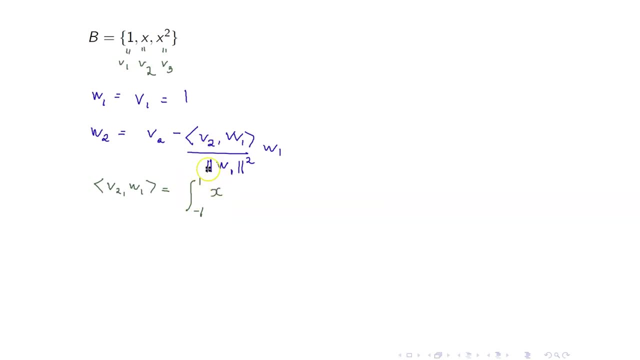 v2 is x. w1 is just 1. this is equal to 0. since this is equal to 0, we no longer have to compute for this. w2 is just equal to v2. next, let us compute w3. w3 is v3 minus inner product of v3 with w1. 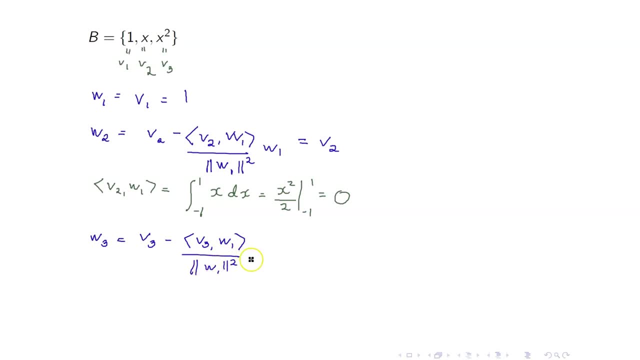 w2 is x. w1 is just 1 length of w1 squared. w1 minus v3, w2, all over w2 squared times w2. let us compute v3- w1. v3 is x squared, whereas w1 is just 1, so therefore this is equal to 2 thirds. let us compute w1 squared. w1 squared is the integral of. 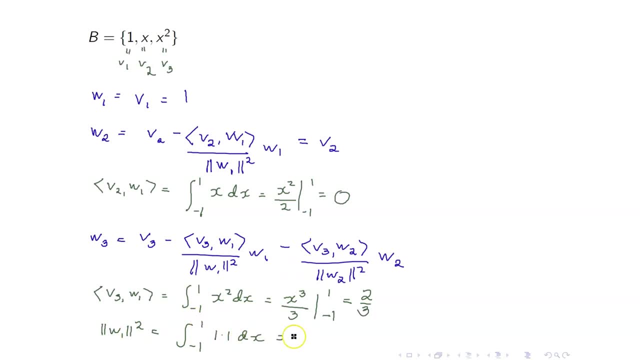 1 times 1, this is equal to 2. next let us compute v3- w2. this is the integral of x squared times. w2 is equal to x and this is equal to 0. so therefore, our w3 is equal to v3 and v3 is equal to x squared minus. 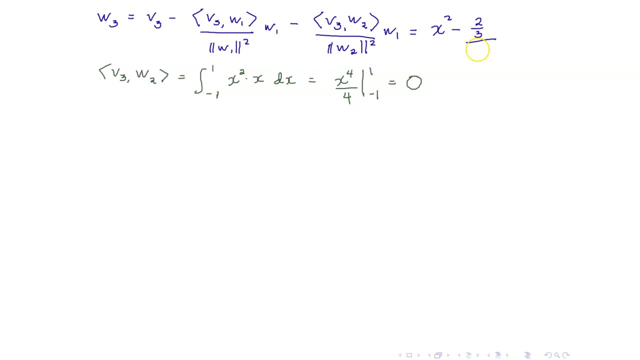 2 thirds, all over 2 times w1, which is equal to 1. so that's x squared minus 1 third. these vectors form an orthogonal basis for p3 using the defined inner product. let us now normalize this to get an orthonormal basis. the length of w1 is equal to square root. 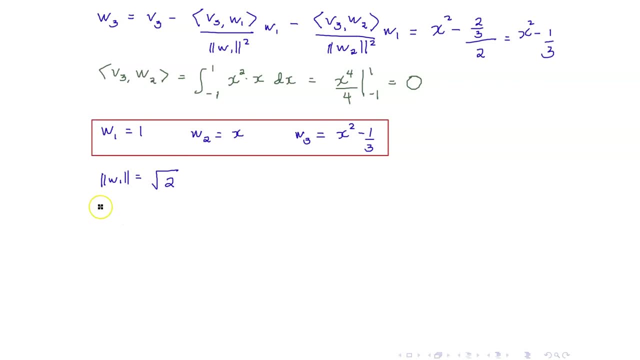 of 2. we've already calculated w1 squared earlier. next let us get the length of w2. this is the square root of the integral of w2 times w2, so that's x squared this is equal to square root of two-thirds. the length of w3 is the square. 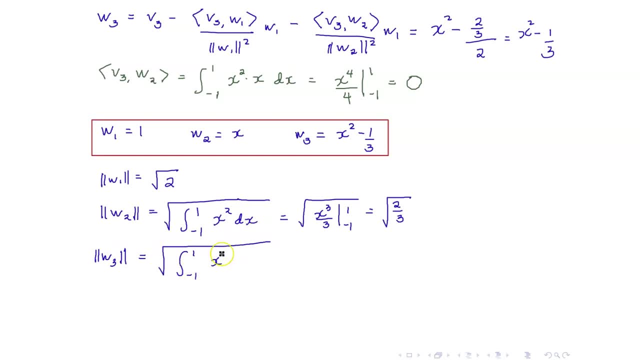 root of the integral of x, squared minus 1 third squared. we're going to, instead of get partialisch and add hatte plus and do that at least so that in the category where you personally own your products, as we say, you don't know beginners but you feel like it's just aว 26 00けれ Hee. like it's 2, 3 square root of 2 squared over 45, which is simply a8 over 45. you could also have u1, which is w1 over the length of w1, which is w1 over the length of w1, is equal to 1 over square root of 2. argues 2 is for square root 8x over and w1 equals 1 over 2x squared is equal to 1 over 2 squared over 50 percent ma lower the oven, universitiesiem.